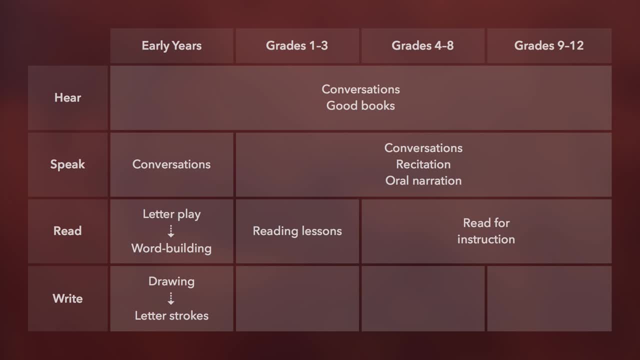 Here are the approximate grade levels that Charlotte used as best practices for language arts. Here are the approximate grade levels that Charlotte used as best practices for language arts. move to paper and pencil. he'll already know the correct strokes Once he has learned to write his letters. you progress naturally to what Charlotte. 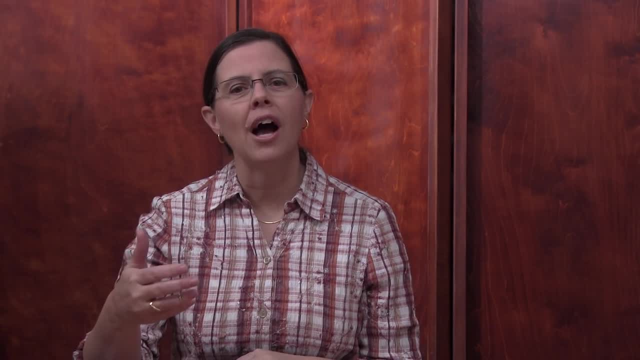 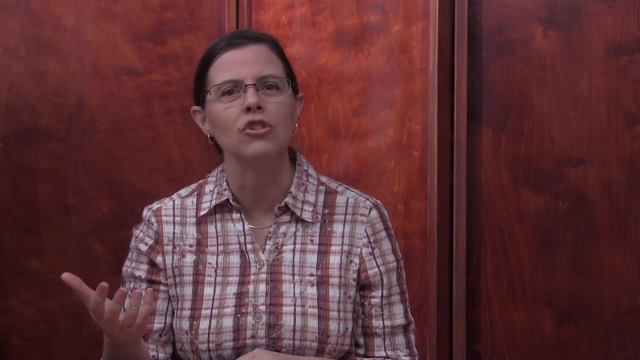 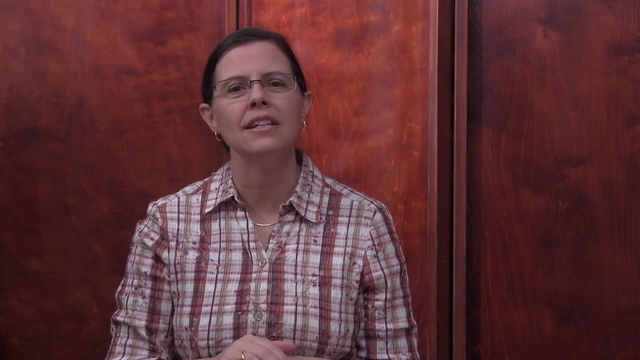 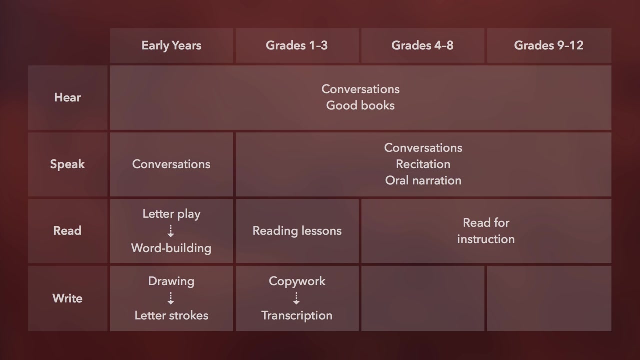 called copywork. Copywork is giving a child words and sentences to copy Passages from beautiful poetry, scripture, quotations or good literature, Being careful to keep the lessons short and to feed his mind with living ideas. Copywork naturally progresses to transcription. Copywork is usually 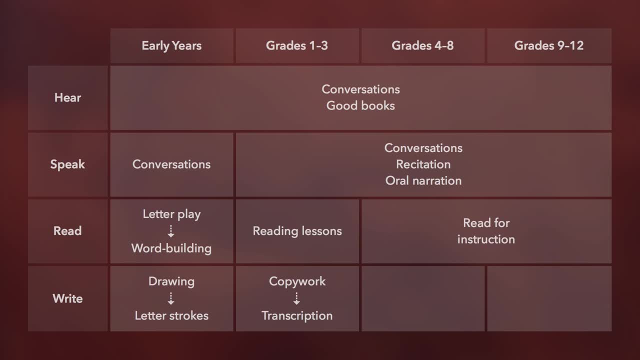 accomplished by copying the model letter by letter. Eventually the child progresses to copying word by word. He looks at a word, gets a mental snapshot of that word, then looks down and writes it. After that he progresses to copying phrase by phrase. When he gets to that stage he's doing transcription and 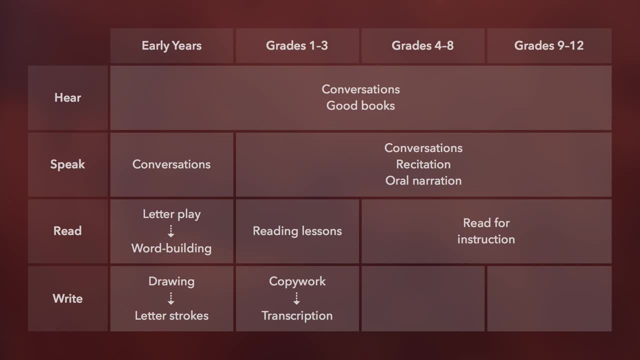 transcription. Transcription naturally leads to the next step: dictation. Charlotte used all three of those methods- copywork, transcription and dictation- to teach spelling in context with great literature, rather than using spelling lists. With dictation, the child looks carefully at the entire passage, but you don't require 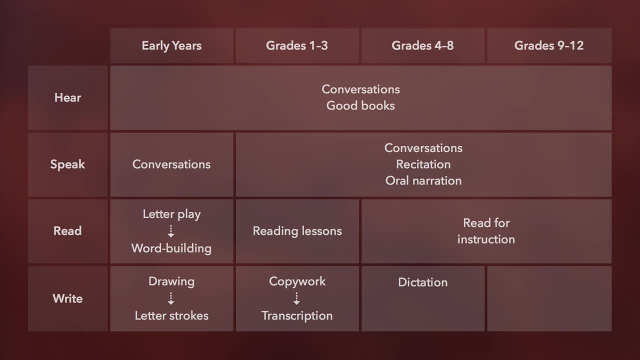 him to write the whole thing from memory. When he is sure he can write it all correctly, you dictate it to him phrase by phrase as he writes. Along with this transition into being comfortable reproducing longer passages, you also ask him to write longer passages in his own words. written narrations. 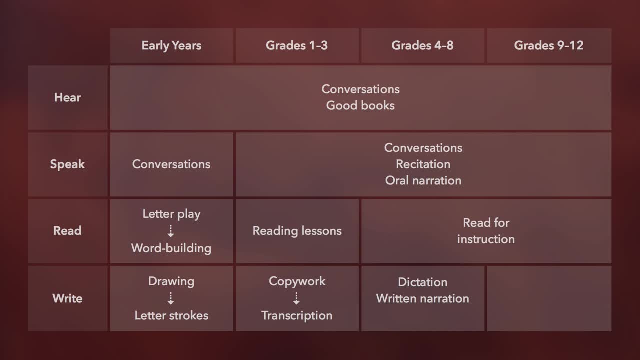 The child has had years of practice with the mental process of narrating because of his oral narrations. Now he simply starts to write somebody. The next natural step is to move into helping the child fine-tune his writing. Now there is a reason to study the parts of speech and how they can affect sentence structure. 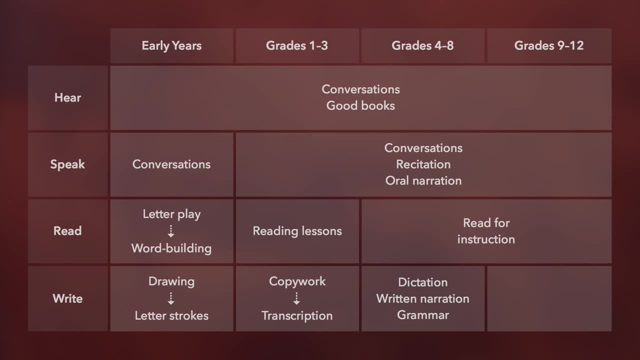 and meaning. As he continues to progress in his writing skills, he has a reason to desire help in his thoughts more clearly and effectively. Notice how those composition lessons can help him structure his life. This can help you with a lot of writing. I have studied Esperanto. 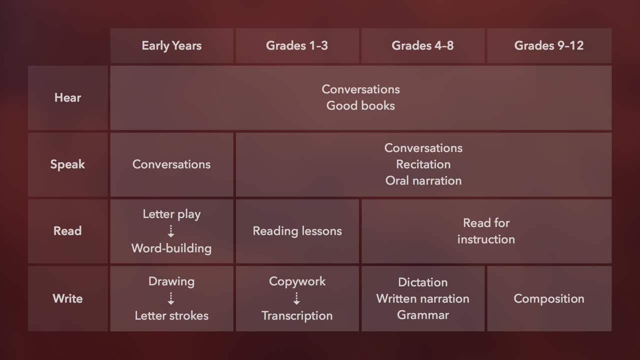 I have learned to write colloquially, So the next natural step is to move into helping the child fine-tune. his writing are a culmination of the natural progression in all of language arts. This fine-tuning is done after the child has spent years. 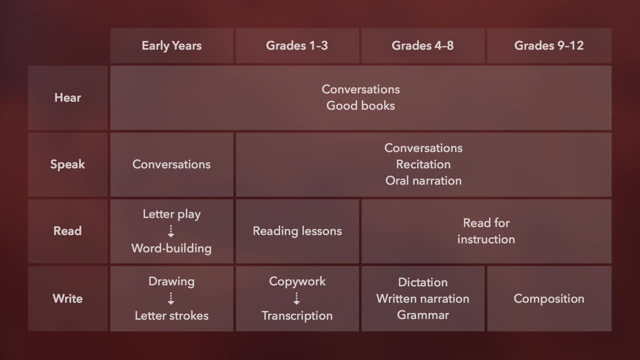 taking in good examples by listening to great books, memorizing and reciting rich literary passages, practicing the mental process of expressing his own thoughts through oral narration, seeing great writing for himself and noticing the mechanics as he reads for instruction, Copying and studying those passages for transcription and dictation. 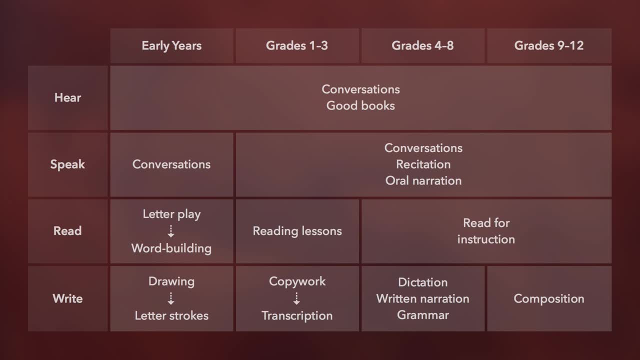 becoming comfortable with handwriting. so the physical action is not a deterrent or an obstacle to expression and developing his own voice from the vast array of excellent authors he has spent time reading and pondering. It is a natural progression toward a multifaceted goal.